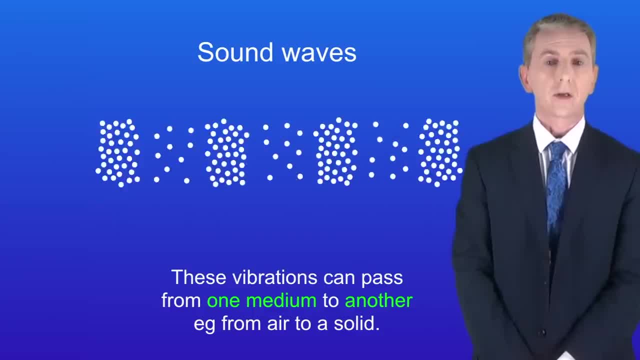 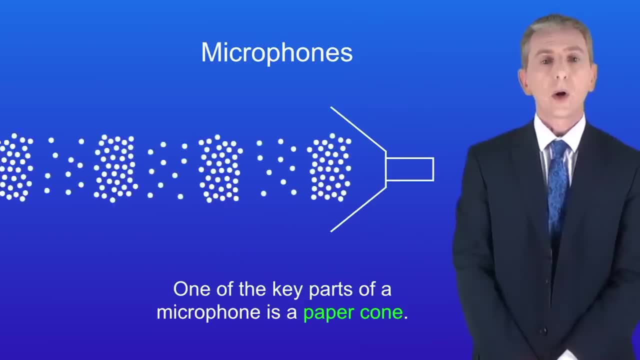 can pass from one medium to another, for example, from air to a solid, And a good example of this is a microphone. We'll be looking at microphones in more detail in a later video, But one of the key parts of a microphone is a paper cone. When sound waves hit the cone, 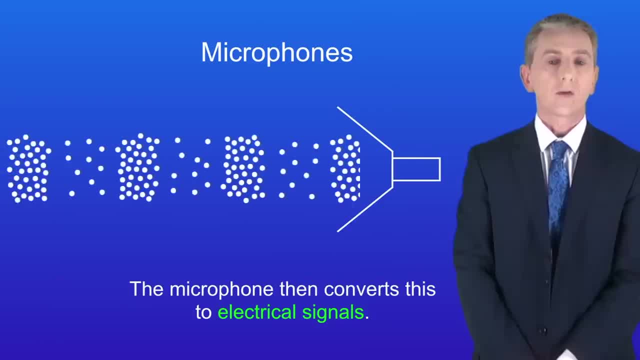 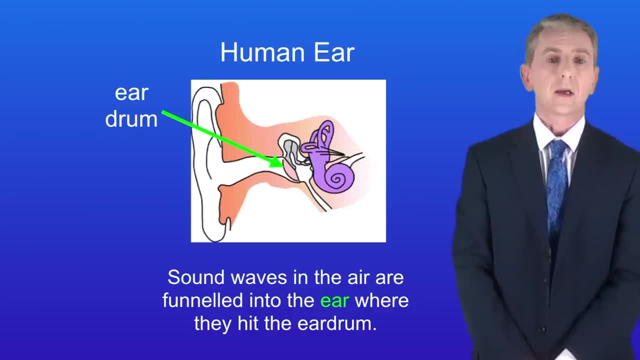 this causes it to vibrate like this. The microphone then converts this to electrical signals. Another good example is the human ear. Sound waves in the air are funneled into the ear where they hit the eardrum, and the eardrum is a thin membrane. The sound waves cause 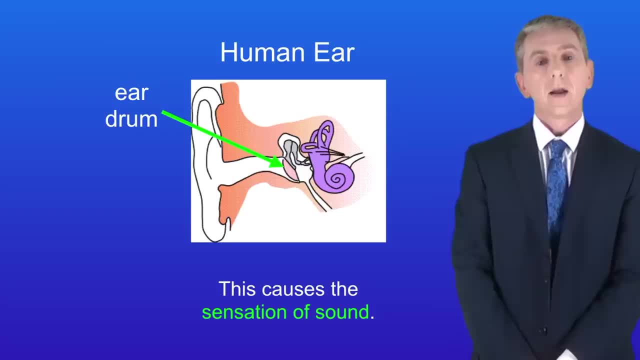 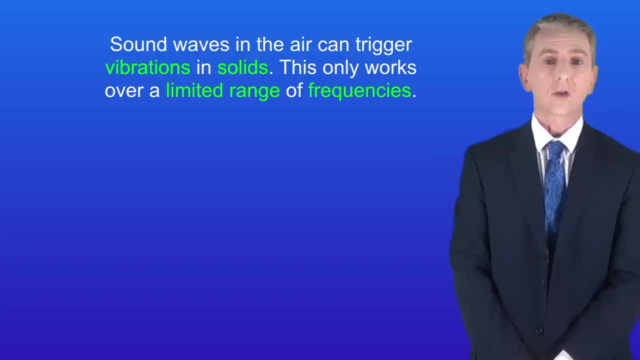 the eardrum and other parts of the inner ear to vibrate and this causes the sensation of sound. So, as we said, sound waves in the air can trigger vibrations and solids. However, this only works over a limited range of frequencies. 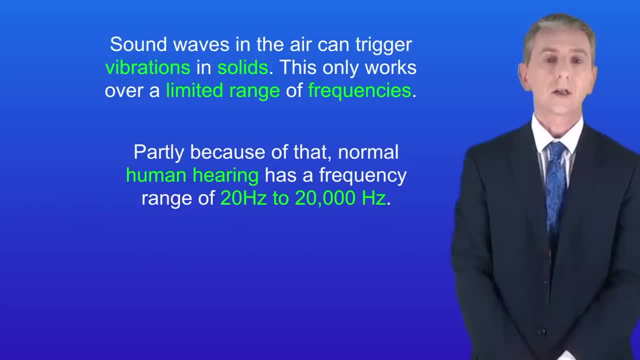 And because of that, normal human hearing has a frequency range of 20 Hz to 20,000 Hz. Frequencies outside of that may not be able to cause the eardrum to vibrate. There is one other idea linked to this that you need to understand. I'm showing you here. 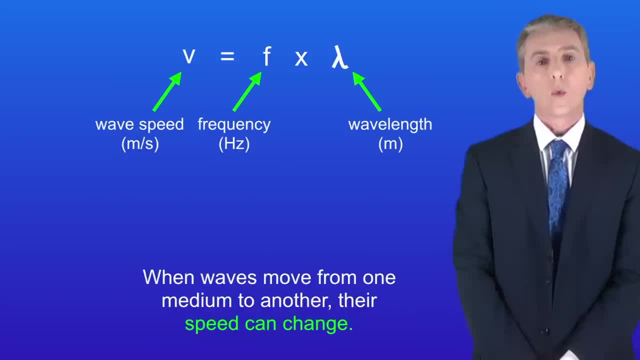 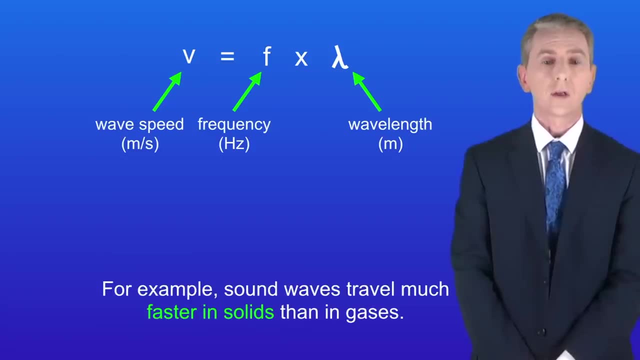 the wave equation, which you've already seen before. Now, when waves move from one medium to another, their speed can change. For example, sound waves travel much faster in solids than in gases. That's because the particles and solids are moving from one medium to another. 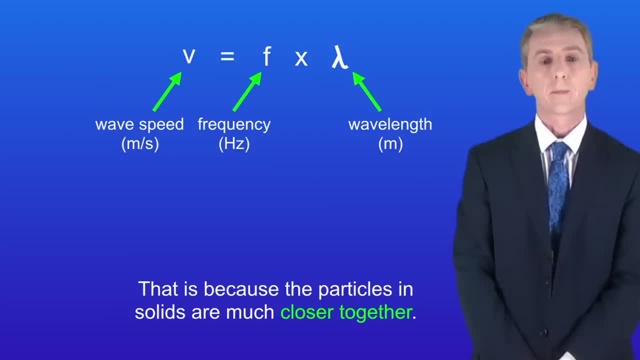 So when the sound waves move from one medium to another, their speed can change. For example, sound waves travel much faster in solids than in gases. That's because the particles and solids are much closer together. This means that vibrations can pass more easily between. 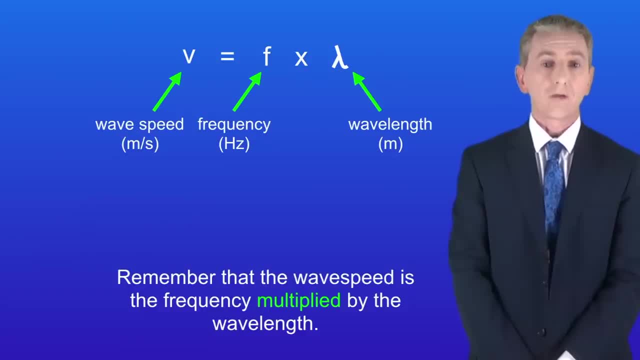 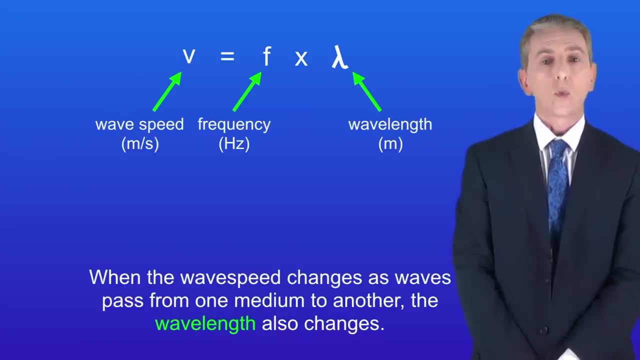 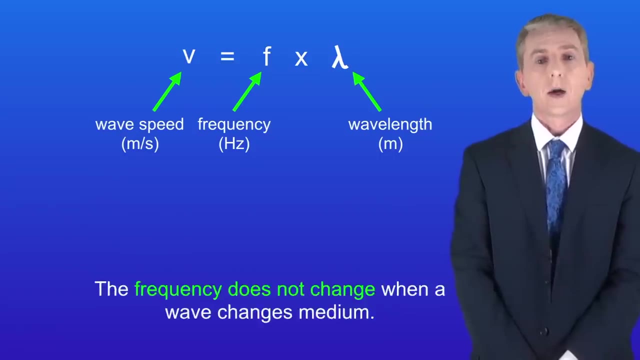 them. Remember that the wave speed is the frequency multiplied by the wavelength. So when the wave speed changes as waves pass from one medium to another, the wavelength also changes. For example, if the wave speed increases, then so does the wavelength. Now I should 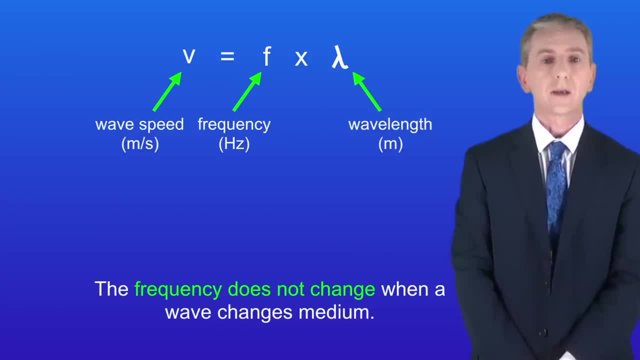 point out that the frequency does not change when a wave changes medium. That's because waves would have to be destroyed or created to change the frequency. So the frequency does not change when a wave changes medium. That's because waves would have to be destroyed. 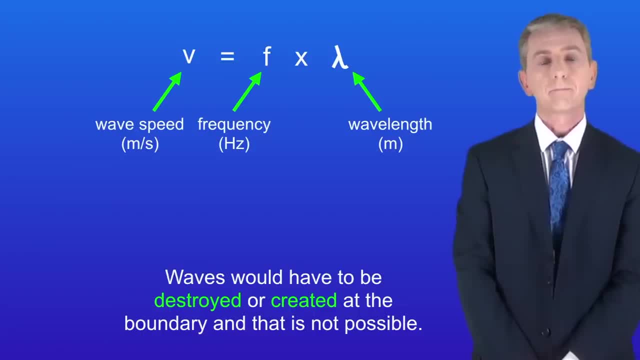 or created at the boundary and that's not possible. And that's because waves would have to be destroyed or created at the boundary and it's not possible at all. Okay, we're going to look now at how frequency and amplitude affect sound. We can view the